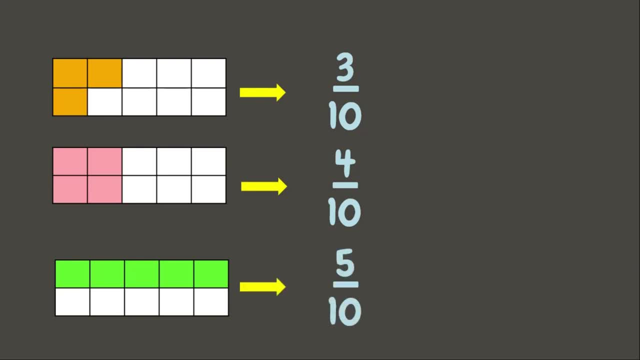 And that is 5 tenths. Great job, But did you know that fractions can be written in another form? Yes, let's have an example: 3 tenths can be written as 0.3.. 4 tenths can be written as 0.4.. 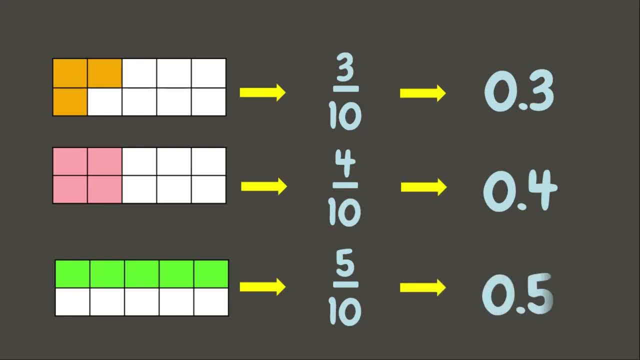 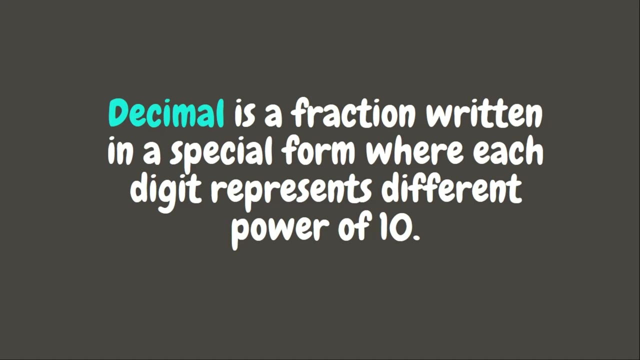 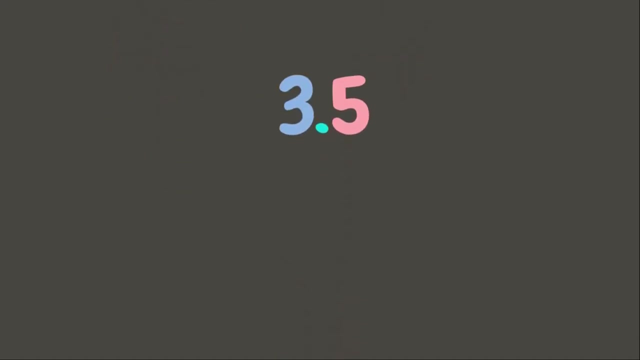 While 5 tenths can be written as 0.5.. These numbers are what we call decimals. Decimal is the fraction written in a special form where each digit represents different power of 10.. Let's have an example: 3.5. 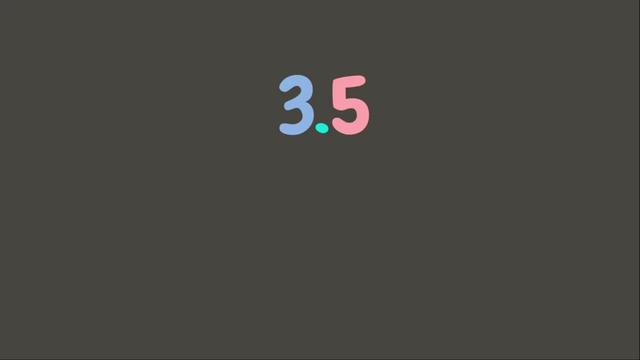 Fractions has two parts. The first one is the number on the left part. They are called whole parts, While the number on the right part is called decimal parts, And the dot between the right and the left side is what we call decimal point. 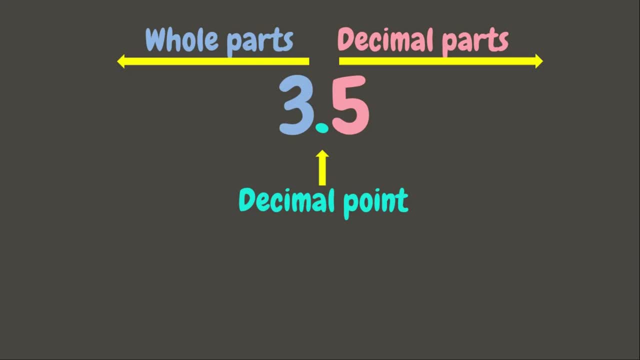 The decimal point separates the whole parts and decimal parts. Now let's have a review of the place values. As we all know, whole numbers have place values. The place value of 3 is ones. If we add another number, the place value is tenths. 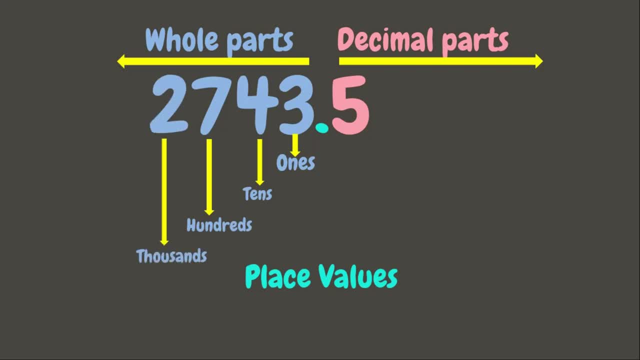 hundreds, thousands, ten thousands, hundred, thousands, million and so on. Decimal part has place values as well. We call them decimal place values. The place value of the first digit on the right side is tenths. The next one is hundreds.